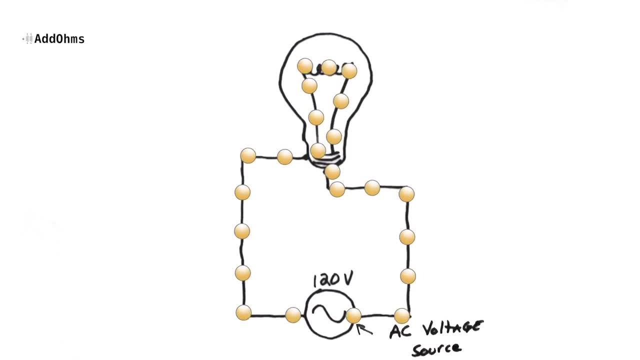 while the current flow was shown as DC. So let's talk about the difference between AC and DC. The letters DC stand for direct current, and it generally means that the electrons flow in a single direction. AC stands for alternating current and it means that the 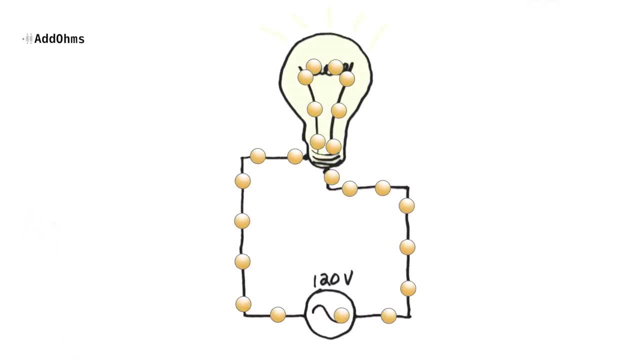 flow of electrons changeNow. this is where things can start to get a little confusing. This is an AC voltage source, so it's both AC and voltage. What the heck? How can voltage and current be the same? Well, it turns out we tend to use AC and DC abbreviations. for voltage electricity sources. So if you are worried about voltage operations, you're right. When trying to change the current you can use an AC source. If you're Efaly, change AC Also over the switch of即. it's a dissipation. you start looking at DC or DC If you're長 blue. as well as current. so in other words, AC voltage or current- is voltage or current? that changes. DC voltage or current: is voltage or current? that is steady, okay. so let's take a little bit closer. look at these two, starting with DC. check out this double a or lr6 battery. it provides 1.5 volts. this example circuit is going. 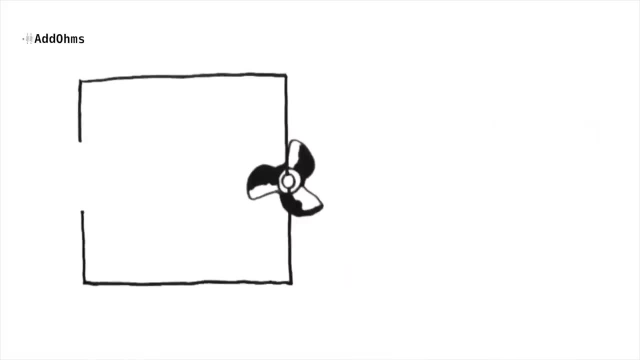 to be a DC motor like you might find in a toy car. when we insert the battery into the circuit, current begins to flow in a single direction: turning the motor. if we drew a graph where the vertical axis is voltage and the horizontal axis is time, we can see that the voltage at this point stays constant. now, since this, 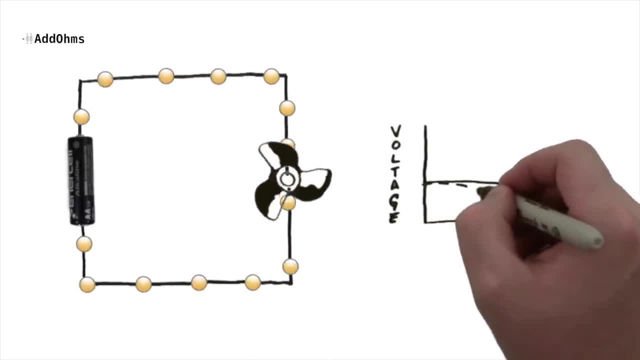 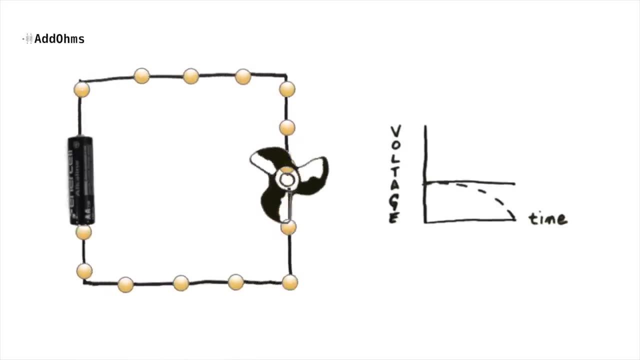 is a battery. eventually it's going to run out of energy and its output voltage will drop. so we know that the voltage will change over time, but the polarity will stay the same. so what is polarity? well, polarity defines the positive direction and, for a battery, the positive voltage. 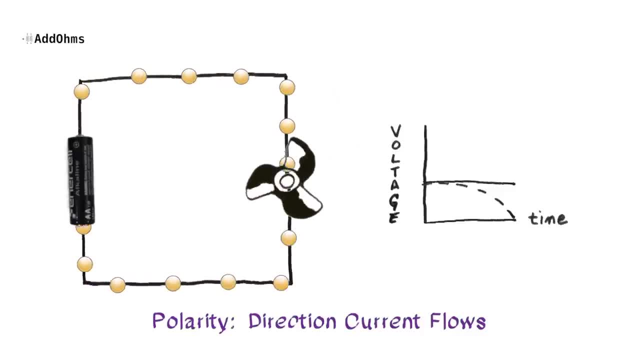 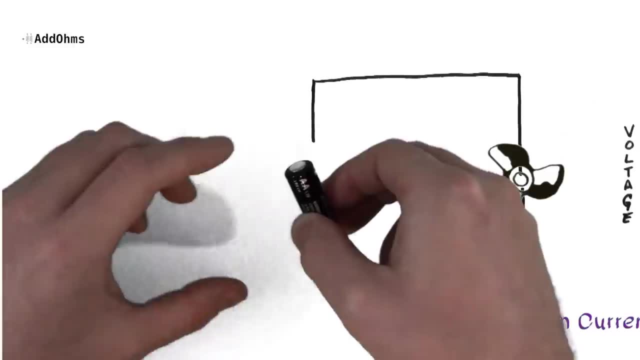 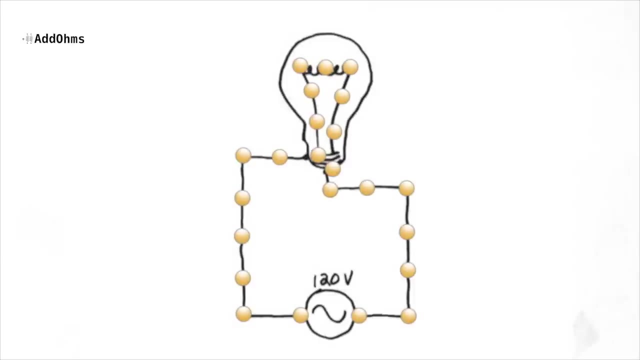 is created from the positive terminal. so what would happen if we turn this battery around? well, that reverses the polarity, which means the current will flow in the opposite direction as before, causing our motor to spin in the opposite direction. okay, so let's move on to AC, and in this case we're going to 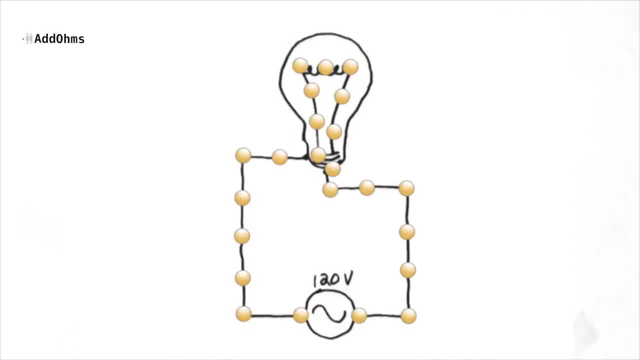 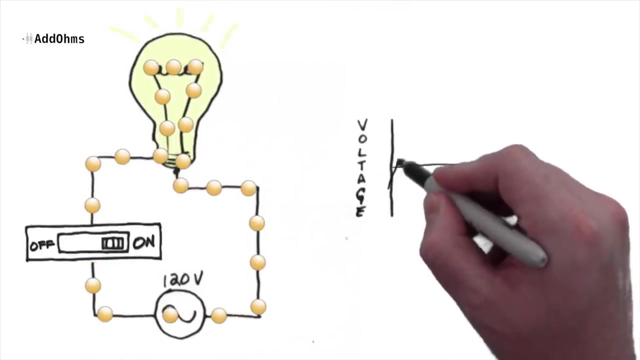 use a light bulb and a North American AC socket, because, well, I live in North America. notice how the circuit behaves when we turn the switch on. let's break down what we're seeing by using the voltage graph. again, notice how the current is flowing in one direction and as voltage increases, the light bulb gets.